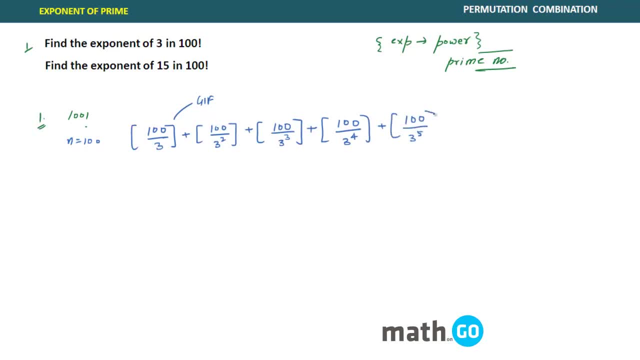 write the next one. It is futile. It is futile to write this also and the further steps also. Why? Because let's see it is 100 by 3 will be 33 point something. So the gif of it, that is, the integer part of it, will be 33. 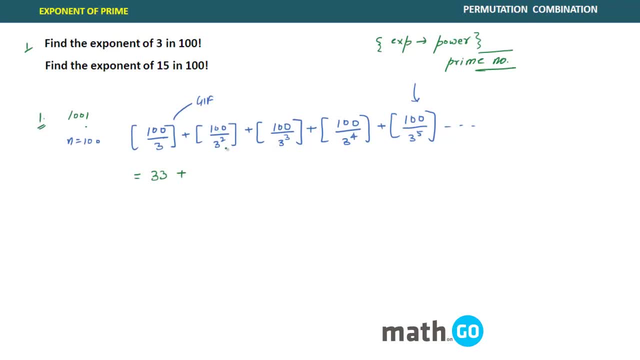 right. This is 100 by 9.. This will give you what 11 is the answer. Only the integer part has to be taken right. So for gif, remember, 11.99 is again equal to 11. It is not round off. It is round off. 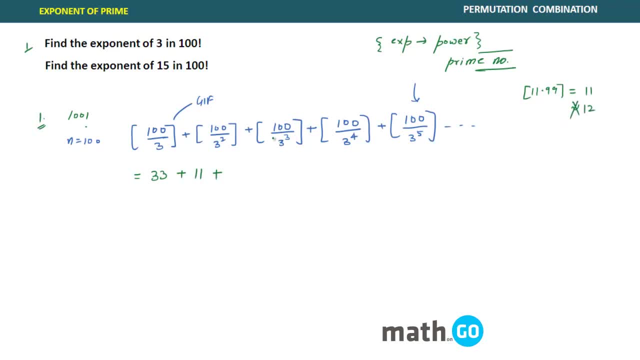 It is not 12.. Believe me right. So this is gif Floor function. This is 100 by 27.. 100 by 27 will have 3 as the equation, 100 by 81. There is only 1.. This will give you 0 and all the subsequent terms will. 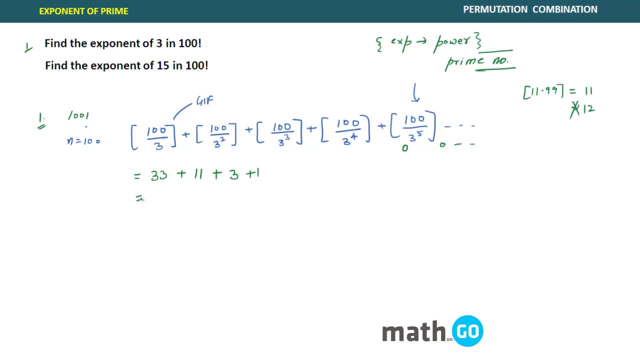 give you 0. So there is no need of writing them, Just add them up. What value will you get? 48.. So that means you will have 3 raised to power, 48 and 100 factorial, So 3 will be there. 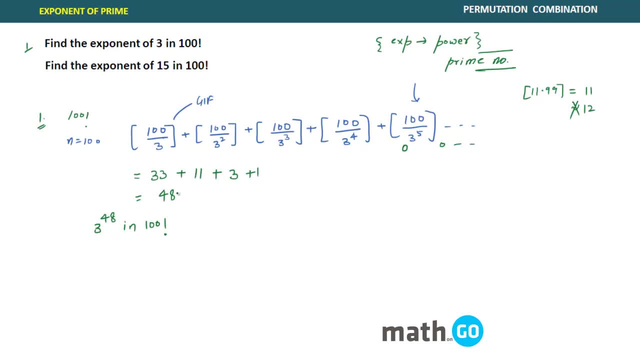 48 times and 100 factorial. that is what is meant by this particular concept And this is how you have to find answers in this. Let us apply this in the second problem. It says: find the exponent of 15 and 100 factorial right. So for 15, how you find 15?? 15 is what. 15 is nothing but 3 into. 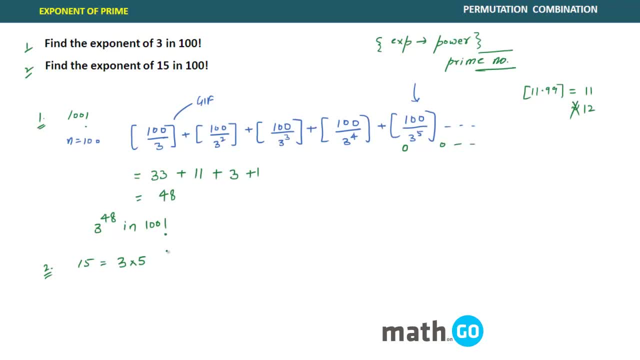 5 right. So you already know what is the power of 3 in 100.. So in 100 factorial right, 3 is getting repeated 48.. 5 is also being a prime. You can also find power of power of 5 in 100 factorial. Let us apply it. 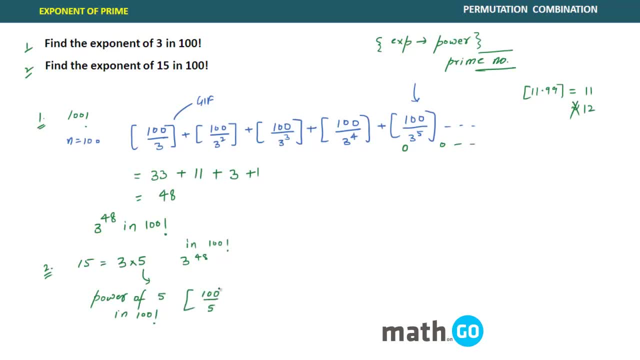 quickly in here also. So it will say 100 by 5 plus, yes, 100 by 5 square, which is 25.. Do you think I have to solve it further? No need, because it will be now 5 cube, which is 125.. This will give me 0.. 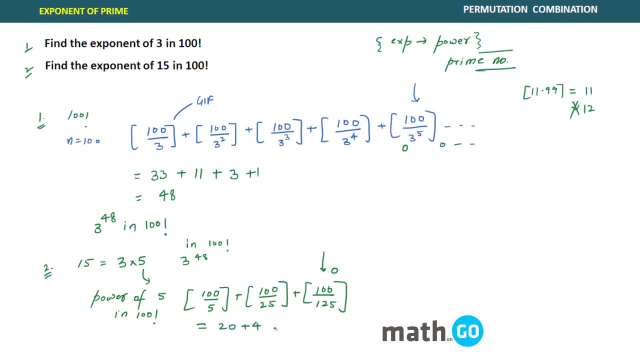 This gives you what? 20.. This gives you 4.. So that means it has maximum power of 5. in this particular number, that is, 100, factorial is 24, right? 3 was there for 48 times, 5 was there for 24 times. So how many times 15 will be obtained? Think, think of it. 3 is: 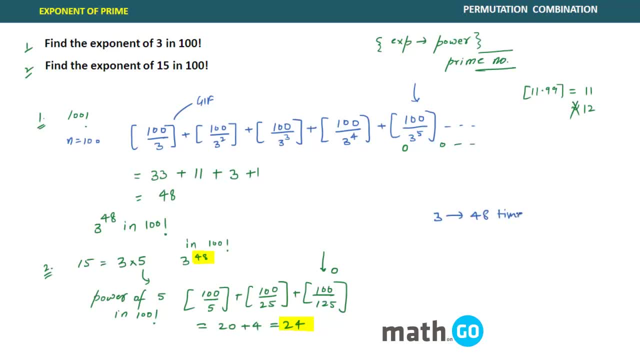 getting 48 times right? 5 is there with you for 24 times, So how many times 15 will be there? Yes, 24 times. Obviously there is a limit, right? So if 5 is limited with a lower value, so that means only that. 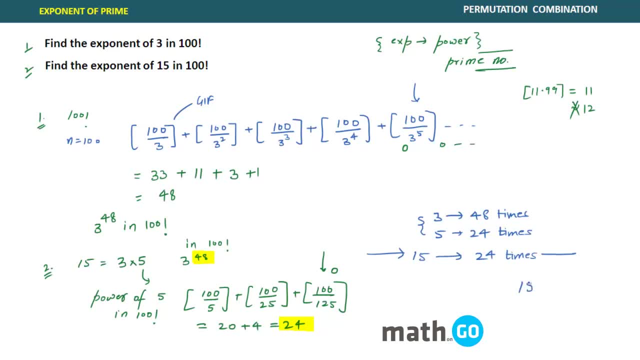 many value 15s, you will obtain So 15.. So that means you will have 15 raise to power, 24 in 100 factorial. This is what is meant by this concept, Brilliant concept. In fact, you will find this concept used in various MBA exams also. Let us take another problem to understand. exponent of a. 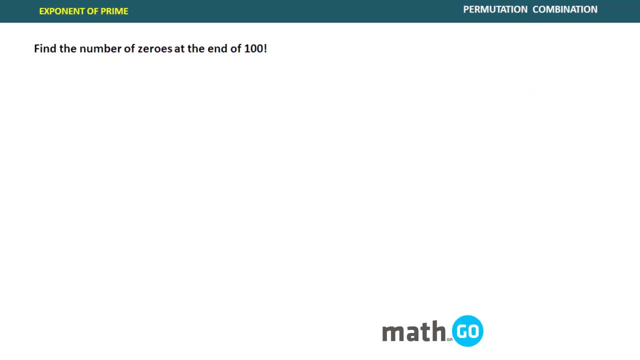 prime. Let us say: let us find the number of zeros at the end of 100 factorial, right? So you need to count number of zeros. What is? when do you get a zero at the end of a number? Yes, when you have a multiple of 10.. So that means it is asking exponent of 10 in 100 factorial. So this is the 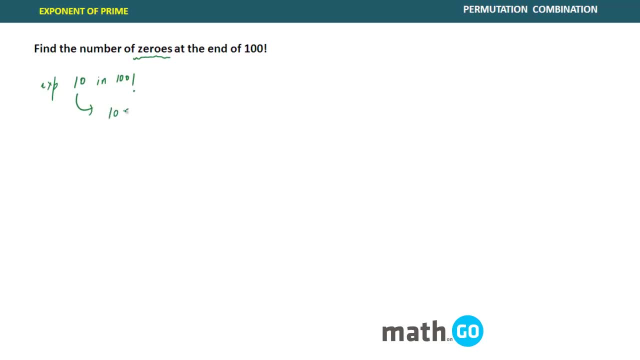 question This is now you people can actually solve. So 10 is obtained by getting 2 into 5.. You have already obtained that. 5 in 100 factorial is nothing but 24 times. We just did in the previous question, right? 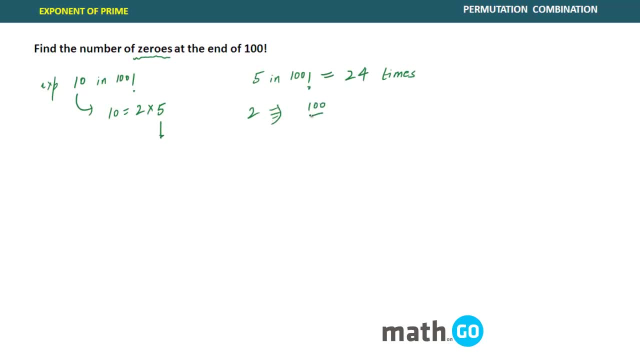 What will be 2? So for 2? let us solve. So 2 will be 100 by 2.. I am just solving, though in fact it is not required. I will tell you why This is by 4.. Similarly, 100 by 8.. Getting it? this is how you solve that, So. 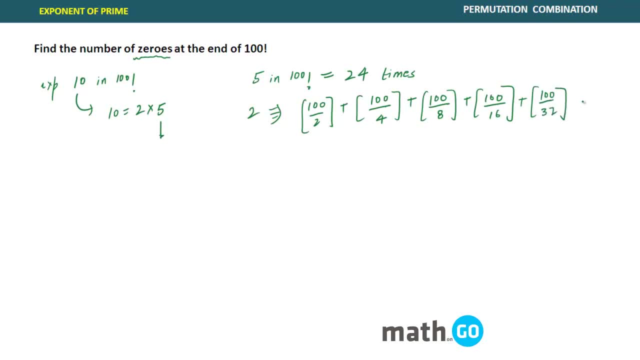 for 2- it is the lengthiest calculation- 32, and this will be the last one, 64.. After that you people will not require, because otherwise it will become zero. So this is 50, 25,, 12,, 6,, 3.. This will be 3 and this.